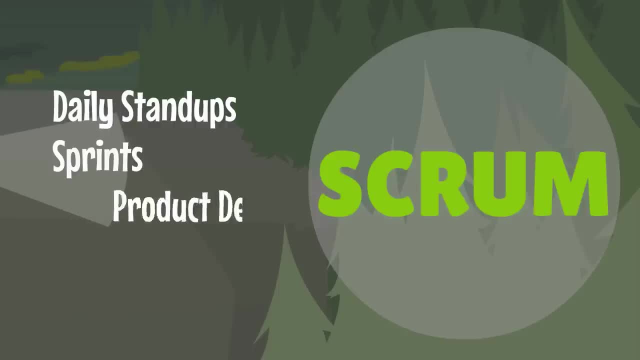 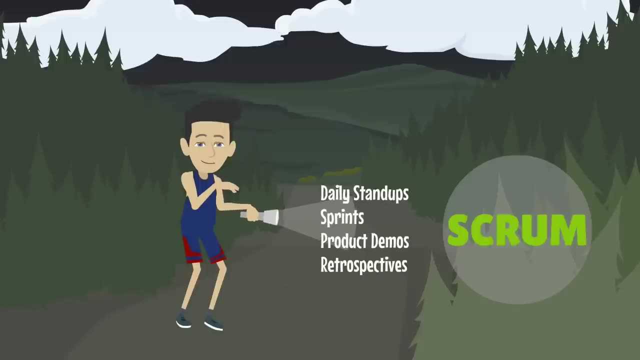 This includes things like having daily stand-ups, fixed length sprints, product demos and retrospectives. Many teams find Scrum to be a very good way of proving catching Agile values and principles. It provides a powerful methodology that assists in following Agile. but it is important to note. 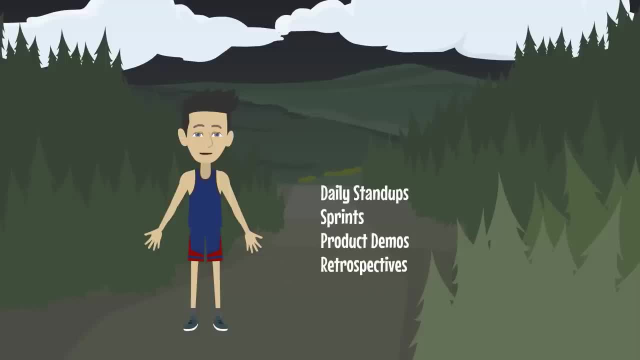 that just following these ceremonies doesn't make a team Agile. That doesn't mean that every Agile team can choose to use Scrum, another method, agile. They have to be following these ceremonies because it helps them align with the agile values and principles. As a side note, some people will argue that Scrum is a framework and thus more. 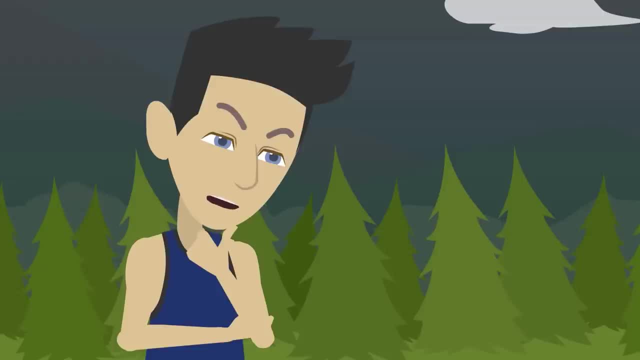 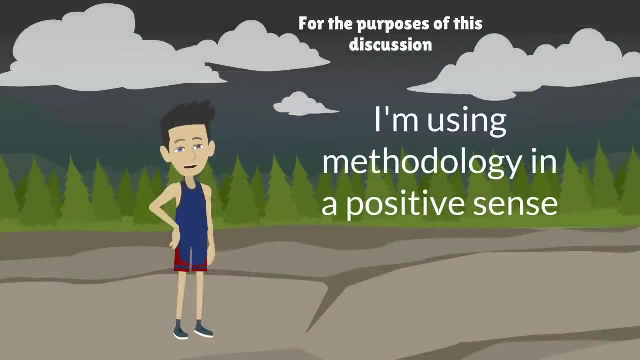 flexible than a methodology, but the line between the two is fairly fuzzy, nuanced and often depends on whether or not someone has negative connotations of the word methodology. For the purposes of this discussion, I'm using methodology, but in a positive sense. Scrum gives you powerful methods. 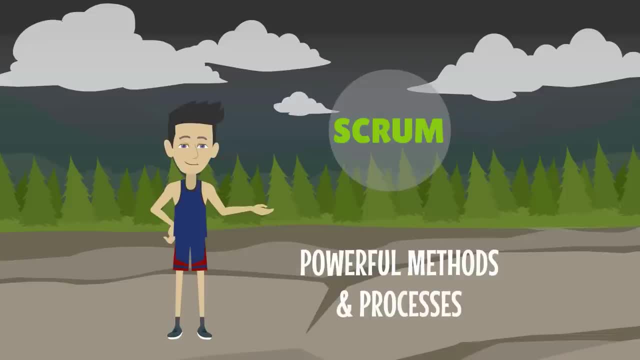 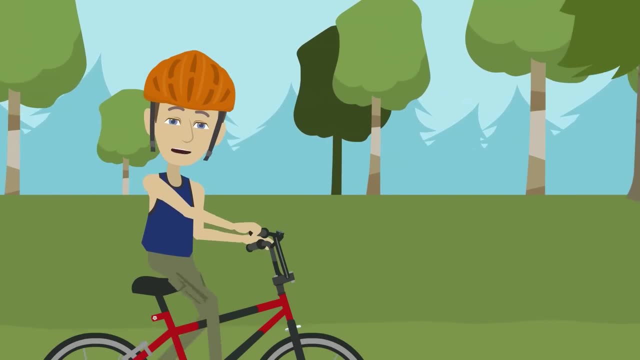 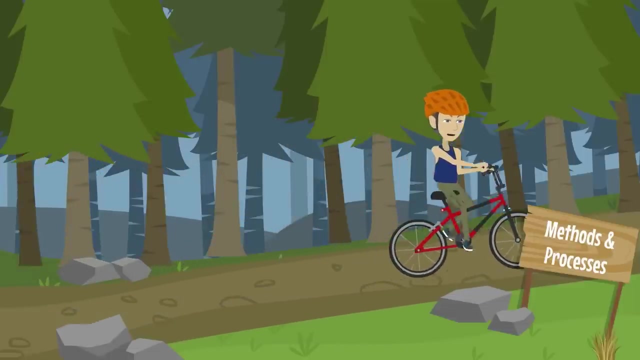 and processes for getting work done. Extreme programming is another methodology that you'll encounter in software development. It includes a number of practices like test-driven development and pair programming. The extreme programming methodology gives teams methods and processes that can be used to follow agile values and principles. For example, agile principles say: 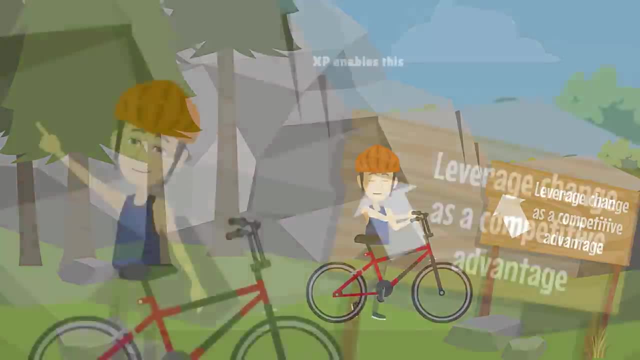 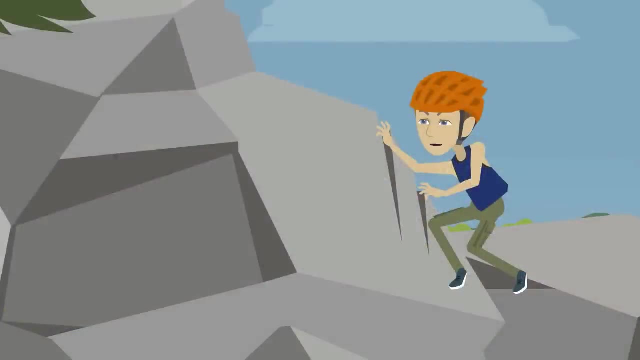 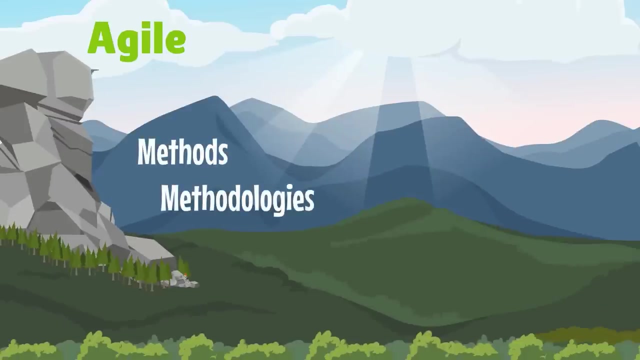 that teams should leverage change as a competitive advantage. XP practices give methods for writing software that enables this. So why do people still refer to agile as a methodology? Usually because they are confusing agile- the values and principles- with the methods and methodologies people use to follow those. 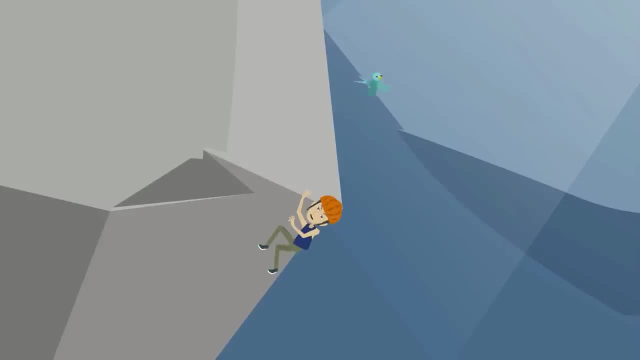 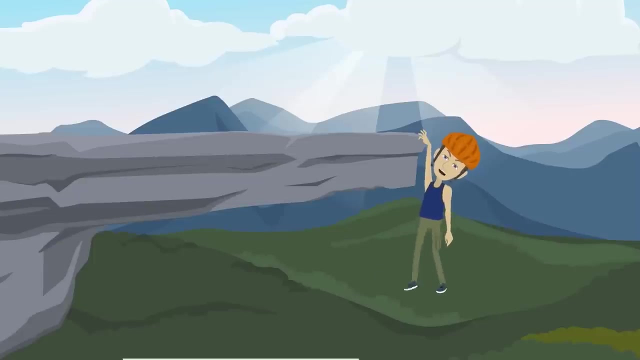 principles. If your team is truly trying to follow agile principles and values, your methodology will evolve over time as your team grows and adapts. After all, that is what it means to be agile. It may seem like a small thing, but every like and every subscription is very appreciated. 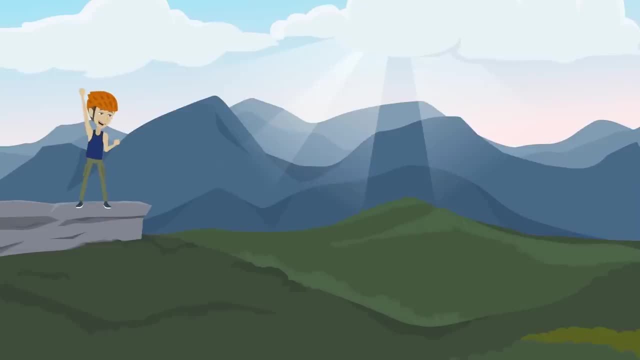 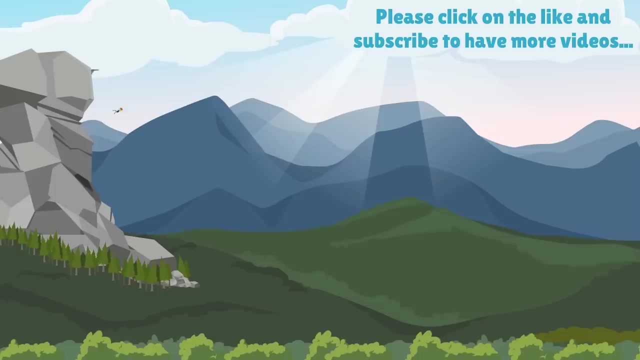 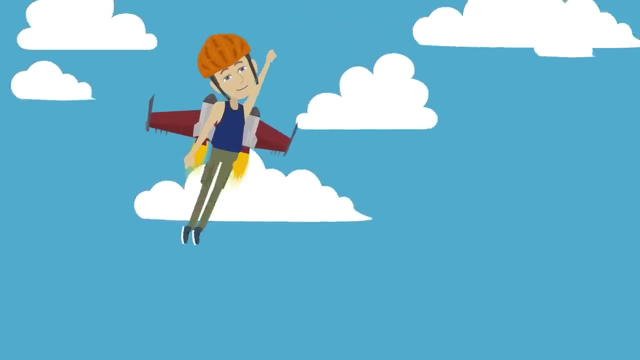 If you'd like to show your support for the creation of more of these videos, please take a few seconds to click on the like and subscribe. If you want to know more about agile, click here for a cartoon explaining the agile principles and values. Also, I have a book on getting started with agile, If you'd like a free.